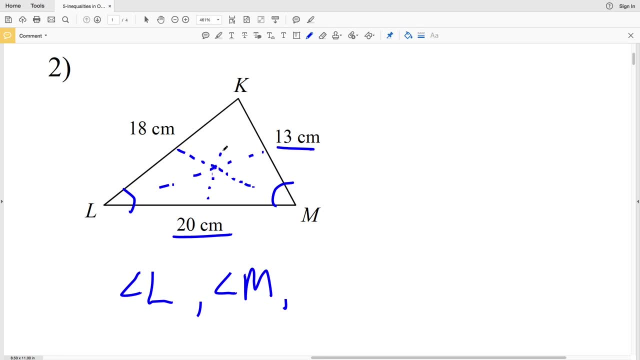 or our longest side is LM of 20 centimeters, which is directly across from 18.. And then our greatest side, which is directly across from K. So angle K is our largest angle. So put an order from smallest to largest: We have angle L, angle M and then angle K And number three. it doesn't give us. 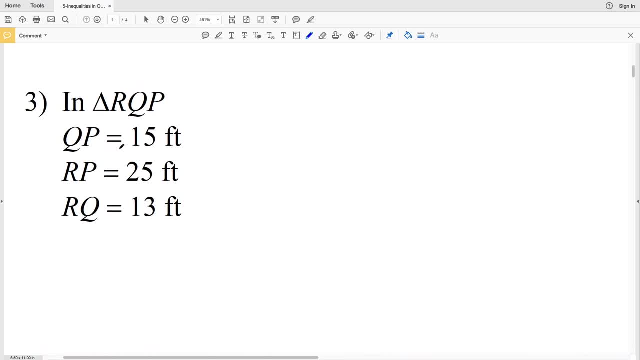 the picture. it just gives us the lengths of the sides. So we have QP, which is 15 feet. So let's say: here's Q, drawing a line, here's P, that is 15 feet. Then we have R to P, which is 15 feet. 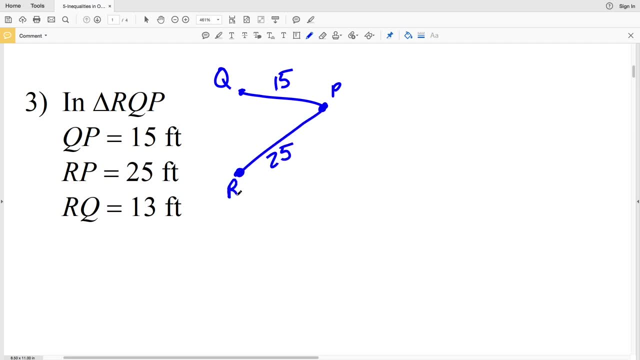 And then from R to Q is 13.. So now that we've drawn our picture, we can easily see from the diagram, since 25 is the largest. the angle directly across from side RP is angle Q. So angle Q is the largest and will get listed last. Next, directly across from our smallest side, is angle P. 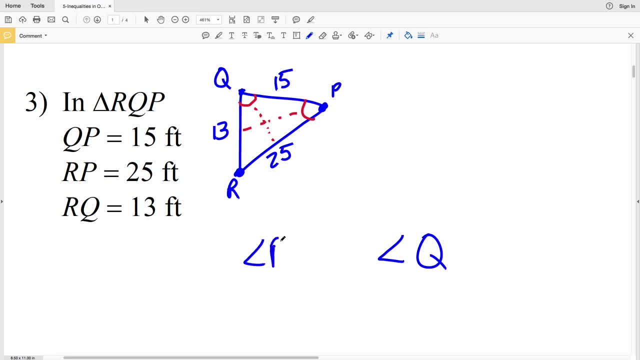 So angle P will get listed last, And all we have left is angle R, which is across from the second smallest side. So, in order from smallest to largest, we have angle P, angle R and then angle Q. However quickly I want to note. 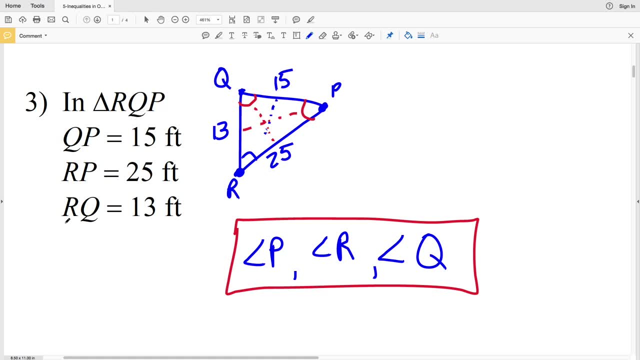 that, since we have triangle RQP, RQ was the smallest side and the angle that's smallest is directly across from RQ. However, looking at our picture, the point left out is P and that's the point of the vertex of the angle. So from this, since we 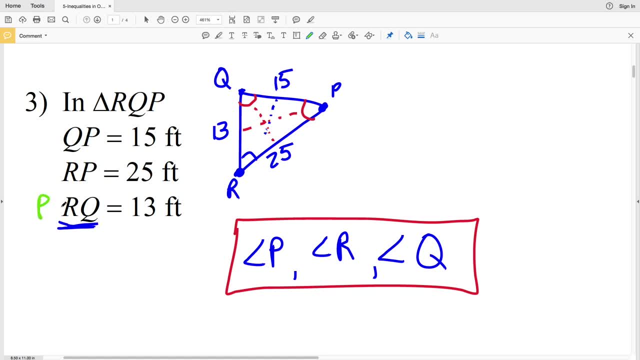 have triangle RQP and P is missing. we know that P is that angle, So P is the angle opposite RQ, Q is the angle opposite RP and the largest, and then R is the angle opposite QP. So we can. 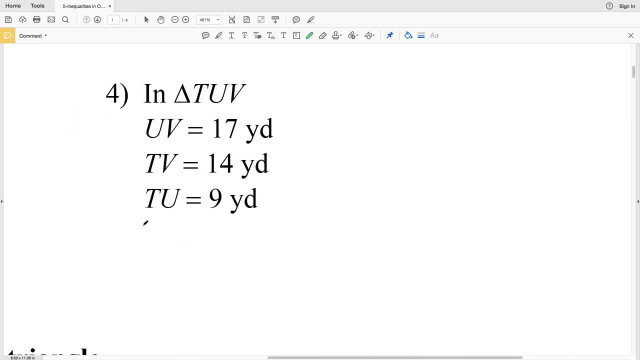 solve this without drawing a diagram. Let's do that in number four. And number four we're looking at triangle TUV. So right away, the angle opposite side UV is angle T, the angle opposite TV is angle U and the angle opposite TU is angle V. So the smallest side is TU of nine yards. Therefore, 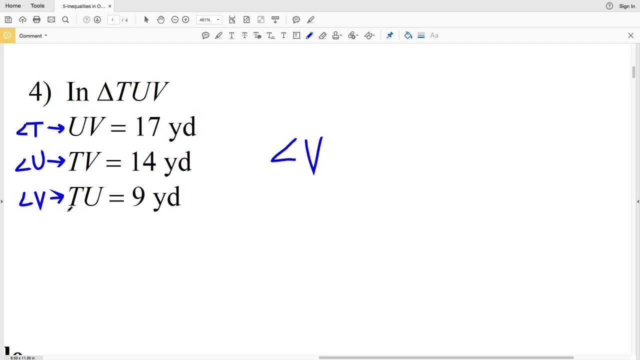 angle V is the smallest angle, the angle opposite that side, The next smallest is 14, since 14 is greater than nine but less than seven. So we're going to do that in number four, And then we're going to do that in number four, And that will be angle U, since angle U is directly opposite angle. 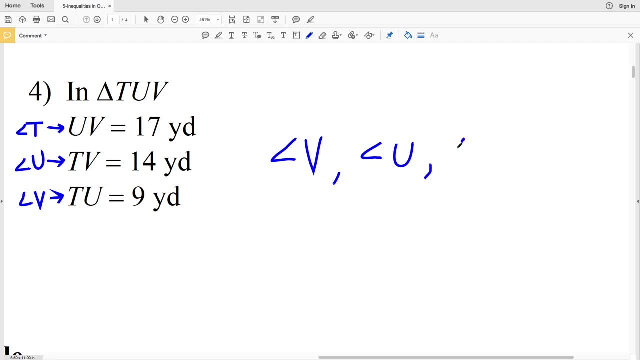 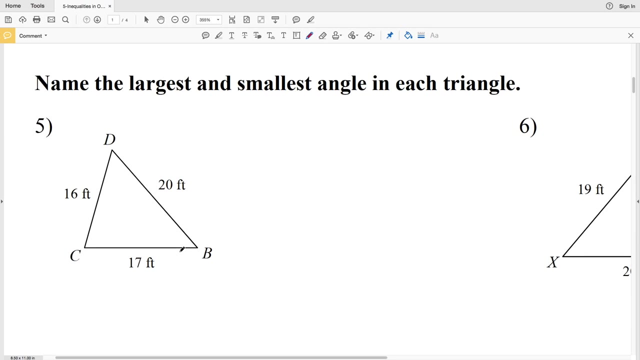 TV And then finally, our last angle, angle T, that's across from the side of 17 yards. So number four, angle V, angle U and angle T is our answer. In number five it says to name the largest and 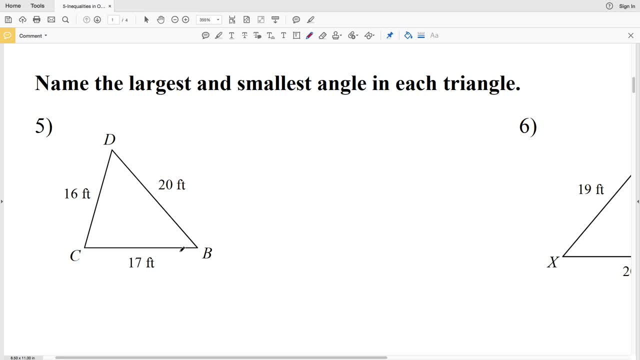 smallest angle in each triangle. So, as opposed to ordering the angles, we're just going to find the largest, least and smallest angle in each triangle. So we're going to do that in number four And then we're going to do that in number five. So, as opposed to ordering the angles, we're just. going to do that in number four, And then we're going to do that in number five. So, as opposed to ordering the angles, we're just going to do that in number five. So, as opposed to ordering the angles, we're just going to do that in number five. So, as opposed to ordering the angles, we're just going to list that first and 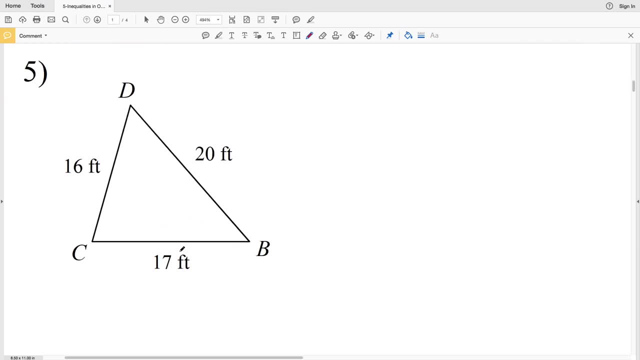 then locate the smallest and list that So in number five, remembering our theorem that the largest angle is across from the longest side and the longest side is across from the largest angle. our longest side is 20 feet. Therefore, our largest angle is angle C, So angle C is the largest. 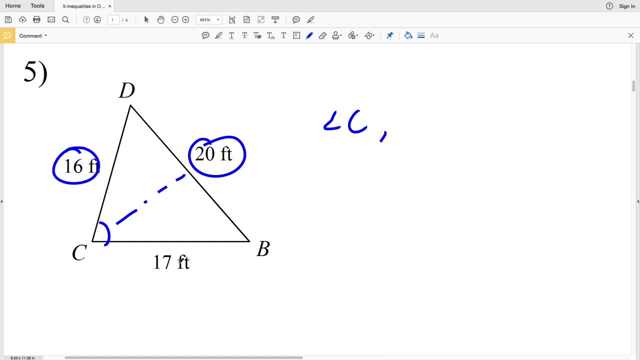 and the smallest is 16, since 16 feet is less than 17 feet, which is less than 20.. And angle B is directly opposite 16 feet. So angle B is the smallest And number six, 20, is our largest side. 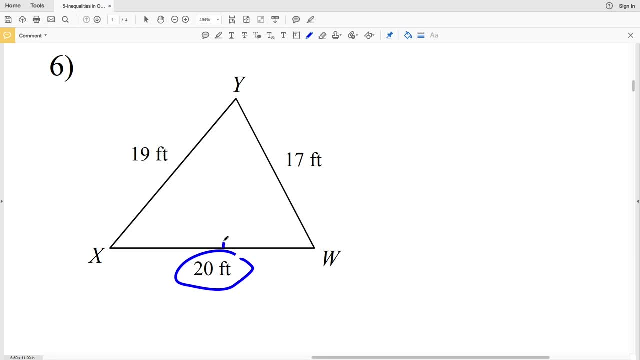 since 20 is greater than 19,, which is greater than 17.. So the angle directly opposite 20 is angle Y. Therefore, angle Y is our largest angle. Then our smallest angle is going to be directly across from 17,, since 19 falls in between 17 and 20.. 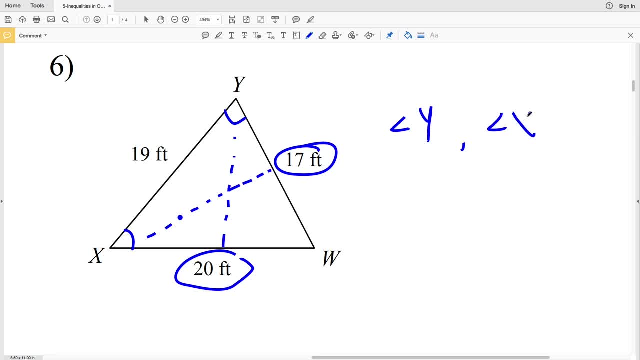 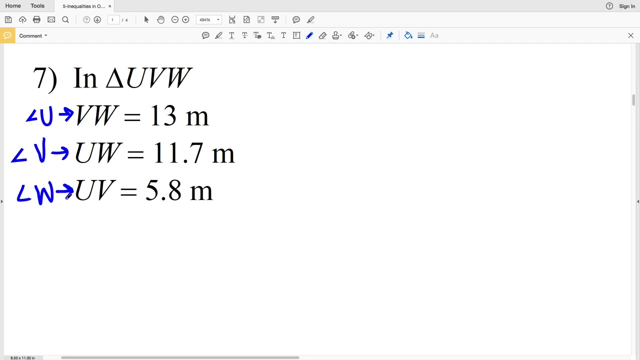 Therefore, angle X is our smallest angle, So angle Y and angle X is our solution. in number six, In number seven, we have triangle UVW. Angle U will be opposite the side VW, Angle V will be opposite the side UW and angle W will be opposite the side UV. The largest side is 13 meters. Therefore,